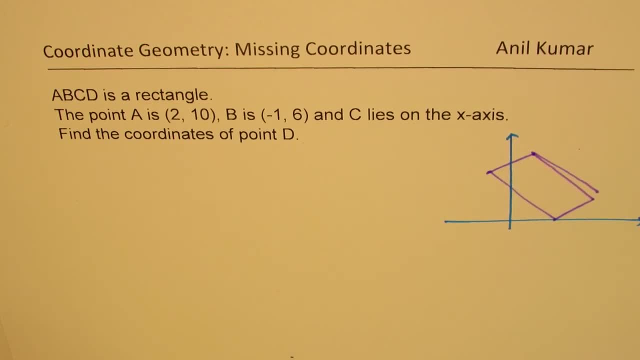 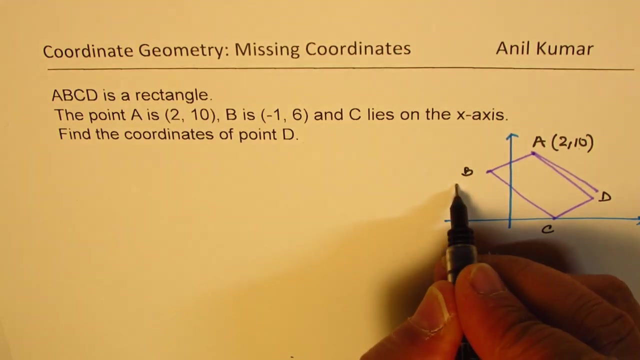 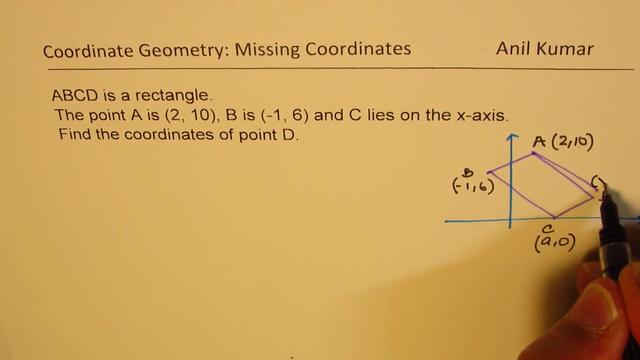 Okay, This doesn't seem like. Let's say this: Okay, So V is an approximate diagram, Definitely not to this scale, But that is how it looks. A is 210.. Okay, A is 210.. B is minus 1 and 6.. C is on the x-axis. So we could write this coordinate as, let us say, x values, A and y value will be 0.. As far as D is concerned, we'll use point x and y. 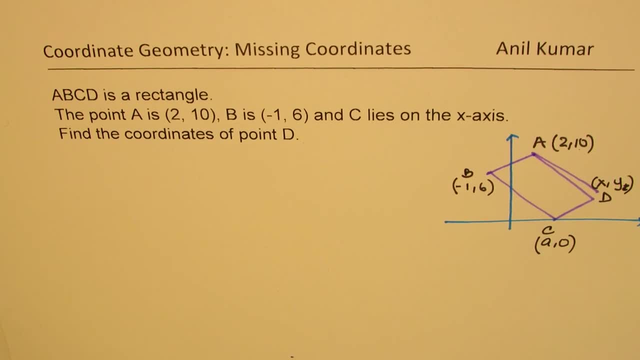 We need to find coordinates of point D. We also know this is a rectangle, So all these are at right angles And these are, of course, parallel. Okay, Now, how do we find these coordinates? Let's first figure out what is C. 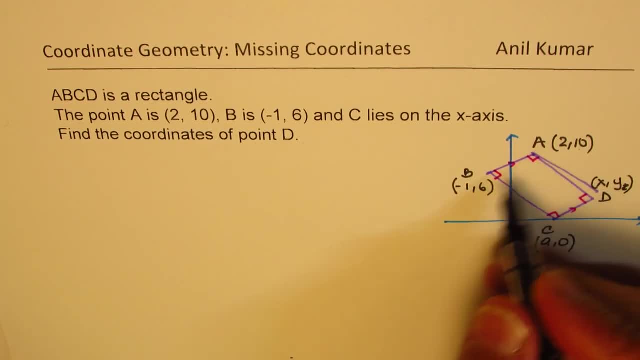 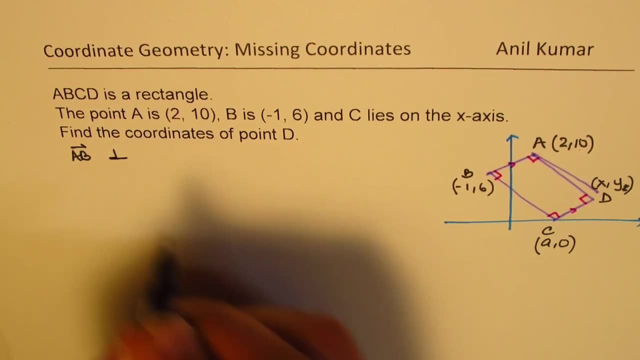 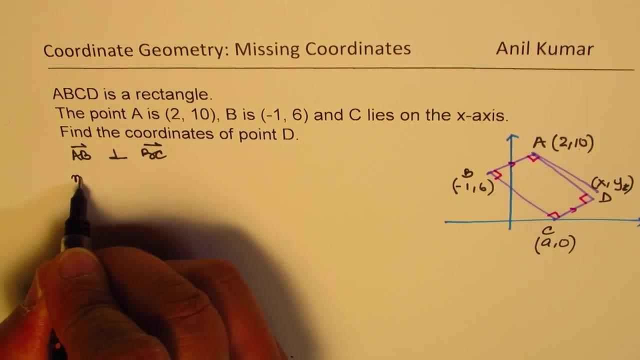 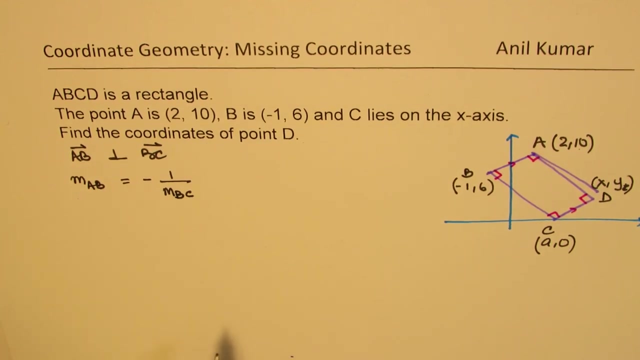 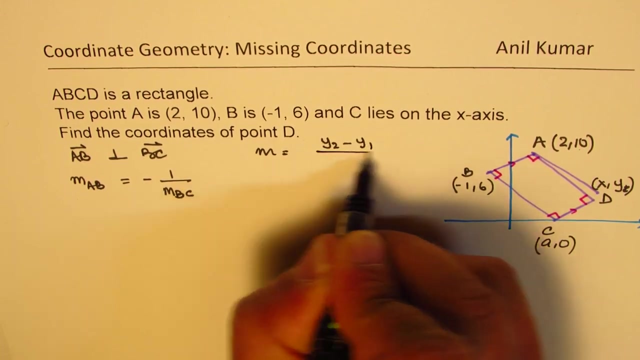 Now we know that AB is perpendicular to BC, Right? So the line AB is perpendicular to BC And that really means that the slope of AB will be negative. reciprocal slope of BC, Correct. So slope of AB is slope in general. M is y2 minus y1 over x2 minus x1. 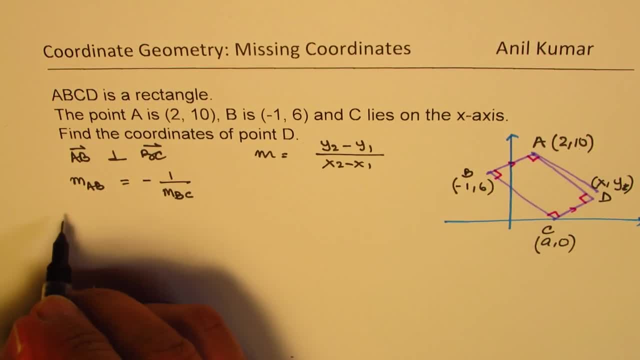 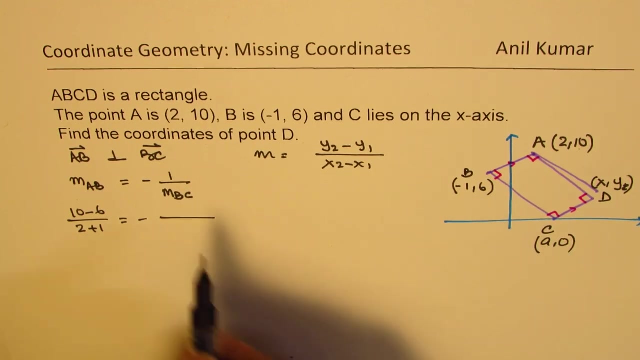 So slope of A to B could be 10 minus 6 divided by 2 minus 1.. So slope of A is 2 minus 1, which is 2 plus 1, and negative M, B, C. slope of B to C difference in y values 0 minus 6.. 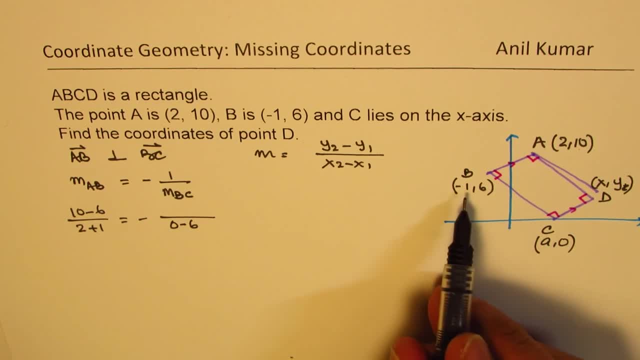 That comes in the denominator. this time, A minus minus 1 means A plus 1.. Correct, So you get this. Okay, So that is what we get. and this ratio on the left side is four into three equals to minus A plus one over x. 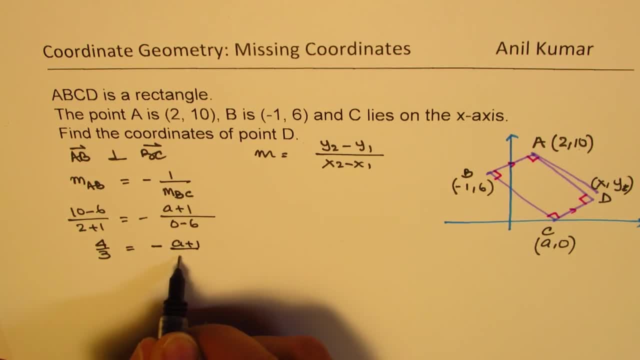 Correct. Okay, So the quotas we get is 2 minus 6, which is 3.. plus 1 over minus 6, so that becomes positive. so we can just make this positive. we can find the value of a just cross: multiply 6 times 4 over 3 equals. 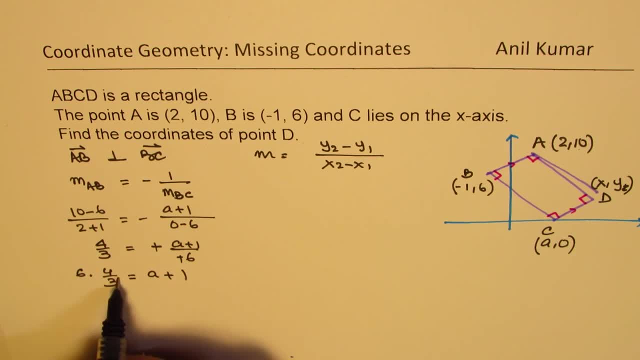 to a plus 1, and this is that goes 2 times. so a plus 1 is 8. so we get a equals to 8 minus 1, which is 7. so we get the coordinates of point C as 7, 0, right so? 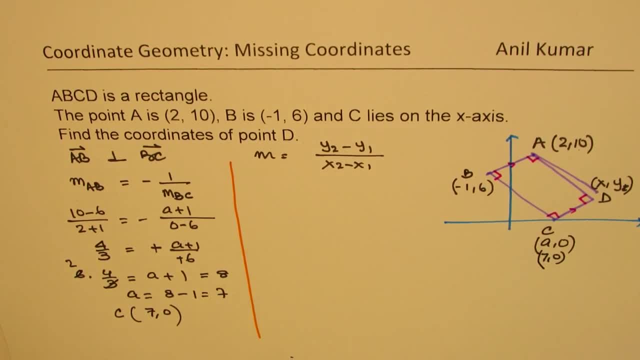 this point basically is 7: 0. now it's easier to find coordinates of point D. we can now equate these two slopes right. so we know slope a- B is equal to slope C to D right. slope a to B we just found is 4 over 3. we're using this value: 4 over 3 right. 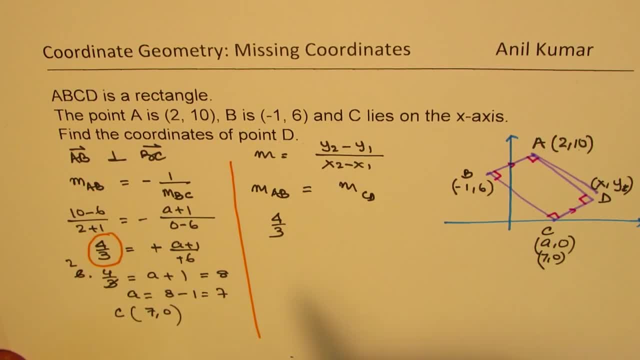 which we calculated that should be equal to slope of C to D. now that is y minus 0. that is y minus 0 divided by X minus 7. now, from here, Y should be equal to 4. that means 4 is equal to Y. we get one value. 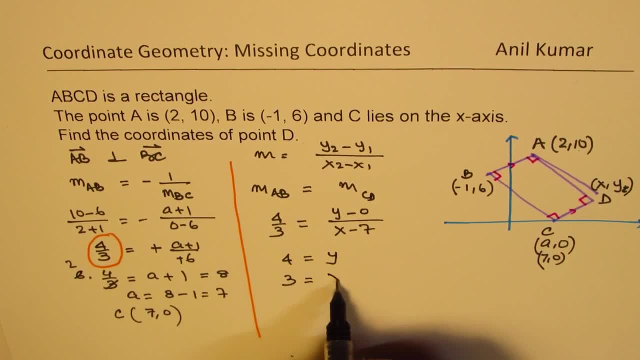 and I'm going to divide that by 4 and use that as Y minus 1 and that's the. As far as x minus 7 is 3, we get 3 equals to x minus 7, or x equals to 3 plus 7,, which is 10, right. 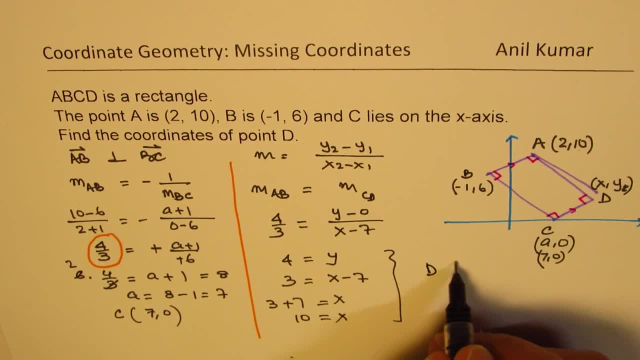 So now we get the coordinates for point D, which are: x value is 10, and the y value is 4, okay, So we get those two points also. So we get y equals to 4, and x equals to 10.. 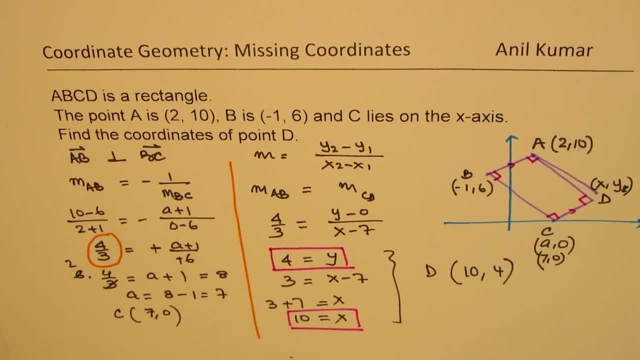 So I hope you understand these steps involved to find this particular solution. So this is a very efficient way of finding the missing points. So what we did was that first we found C by equating perpendicular lines, and then we found C- D, by using parallel lines. 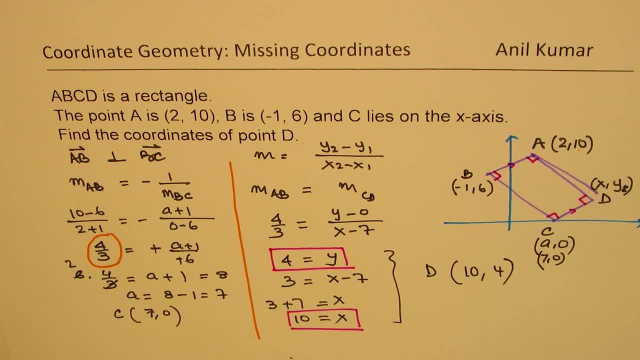 Perfect, So I hope that makes sense. Feel free to write a comment, share your views and, if you like, and subscribe to my videos. that'd be great. Thanks for watching and all the best.